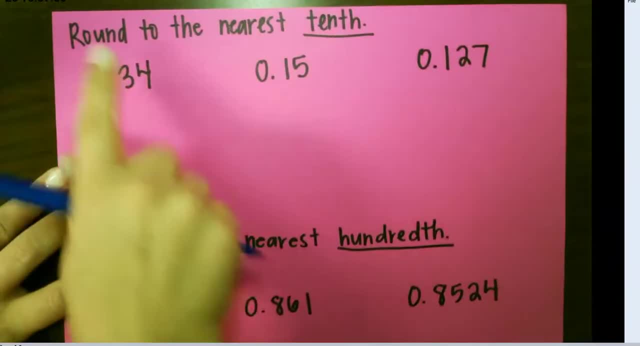 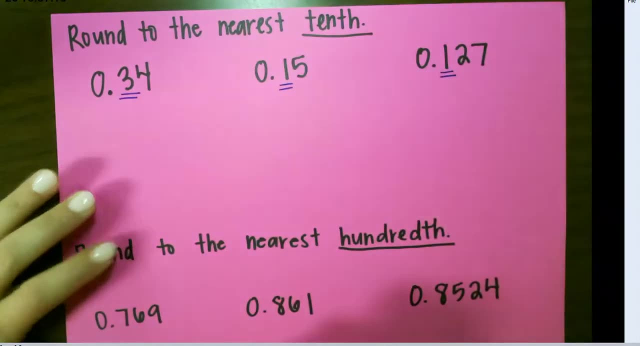 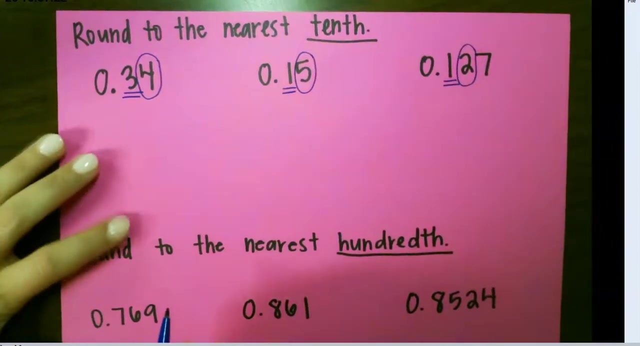 and it will continue going from there. So our first example is: if we want to round these to the tenths place, that's going to be the first number after the decimal. Okay, it is important to note that we need the number right after that as well. Okay, so if it's. 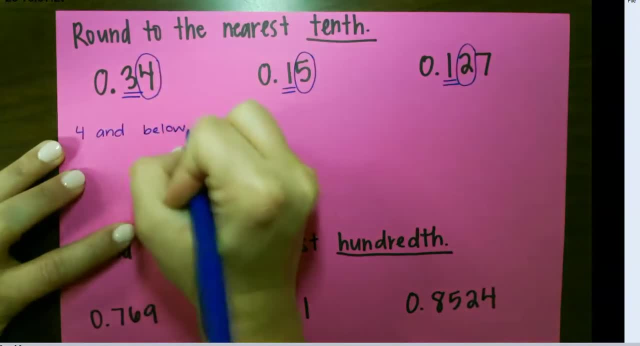 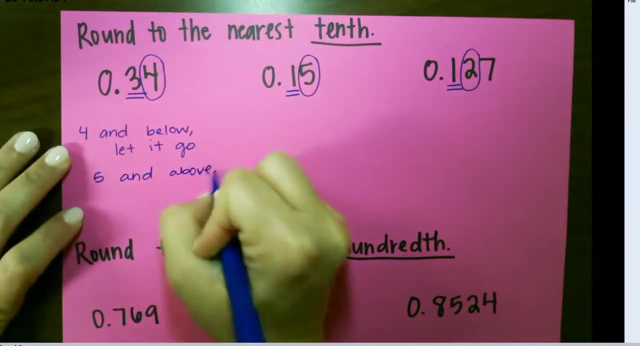 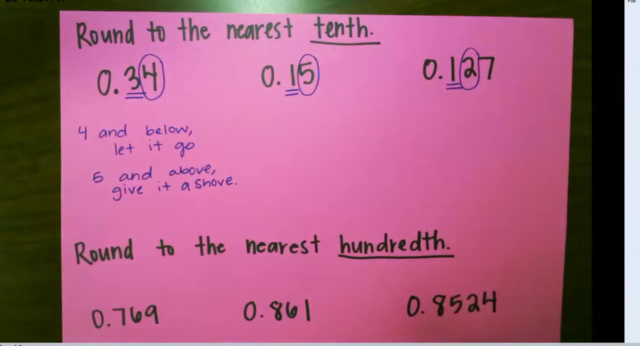 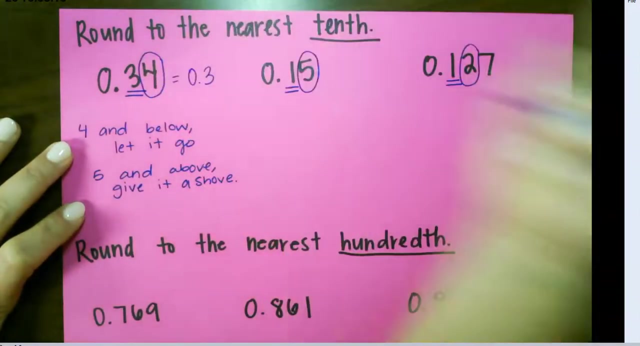 four and below, you let it go, But if it's five and above, give it a shove. That's just a helpful phrase to remember what to do. So on our first one, since it's four and below, we just round this to 0.3, or zero and three tenths For this one. again, the one is in. 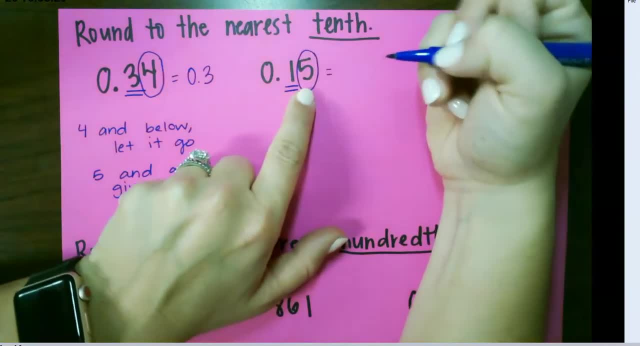 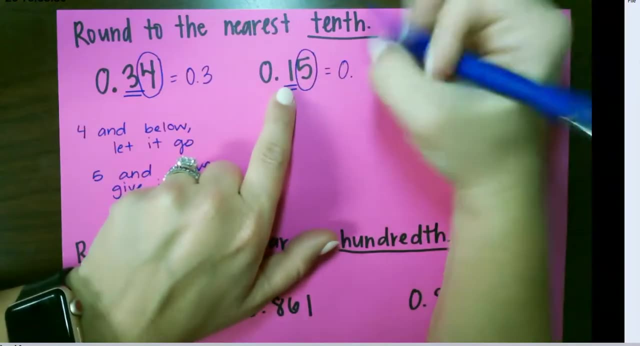 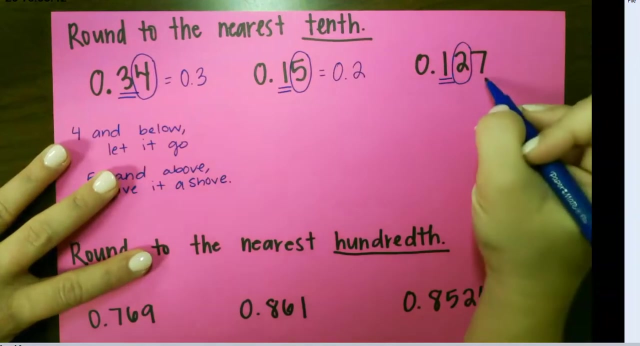 the tenths place, but we need to look at the second number or the number in the hundredths place to figure out how to round this Five and above. you're going to take this number and round it up, So that would be 0.2, or zero and two tenths. For our next one, our 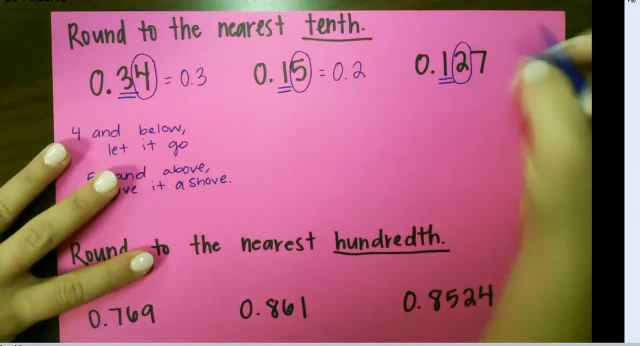 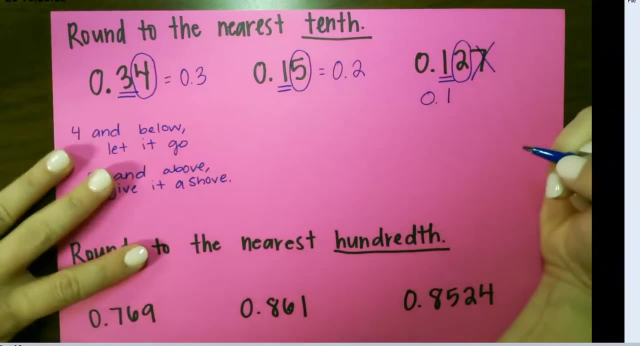 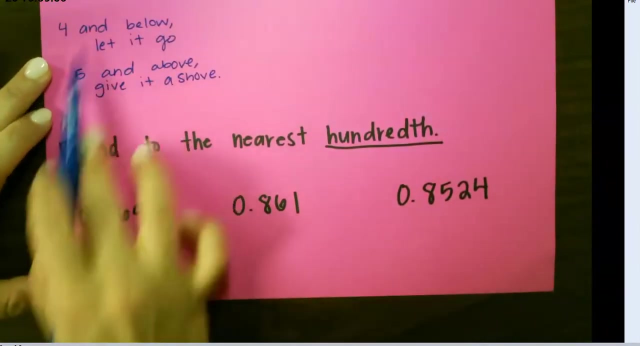 decimal goes all the way out to the thousandths place. but we don't need this number, We only need the two. So it's four and below. so we leave it alone and it just goes to 0.1, or zero and one tenth. Let's look at rounding to the nearest hundredth. This rule still. 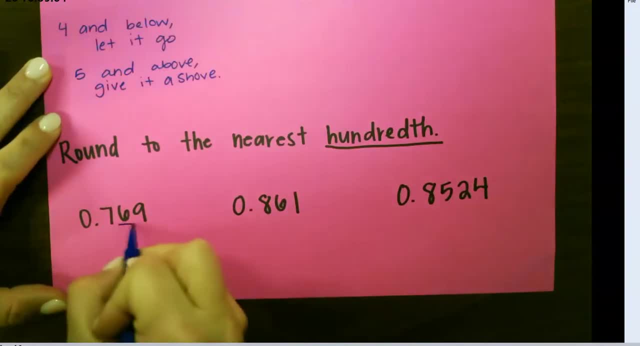 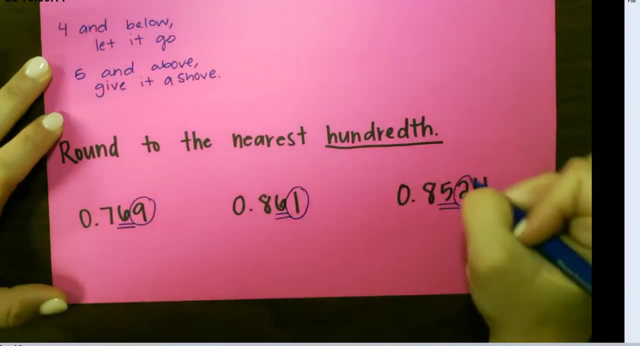 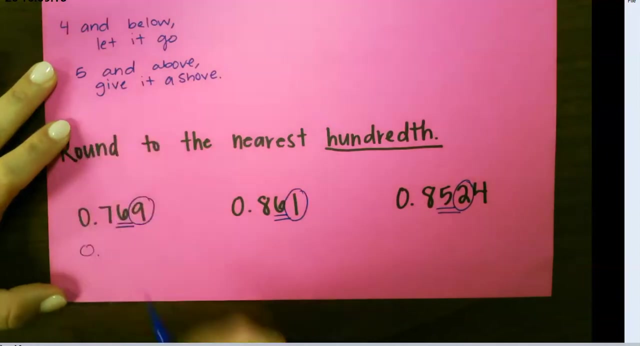 applies. So this time the hundredths place is the second decimal, but we need that third number to tell us how we round. So on, this first one is above 5, so I'm going to round this up to 0 and 77 hundredths For our second. 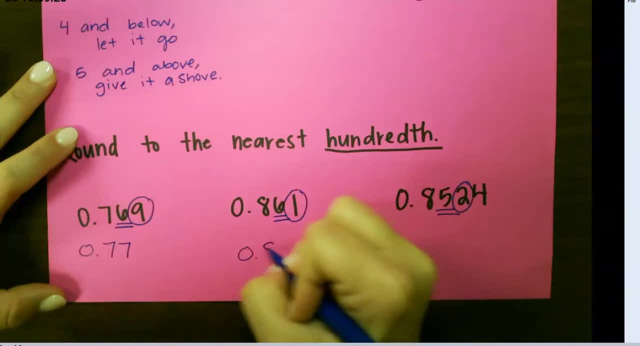 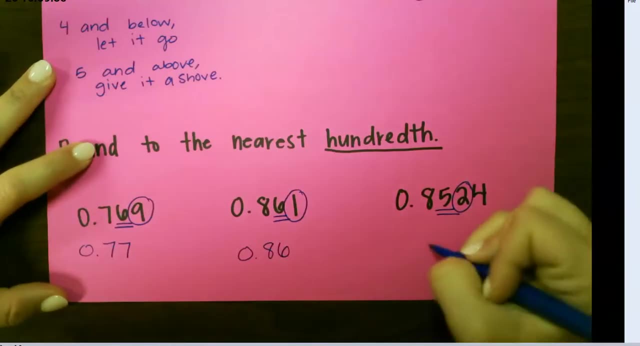 one 1 is below 4, so we're going to leave it alone and round down to 8, 6 or 0 and 86 hundredths. And for our last one, 2, is also below 4, so we leave it alone at 0. and 85 hundredths.